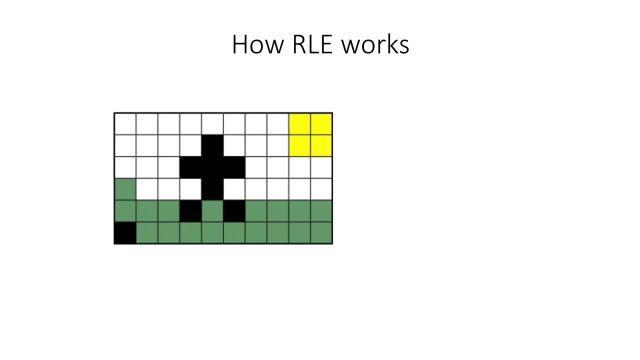 Okay, this is what happens. you have this image and it's got lots of white pixels, then it's got yellow pixels. so if you look at 1, 2, 3, 4, 5, 6, 7, 8 white pixels, and then it's got two yellow pixels, one, two yellow pixels, and if we represent that, 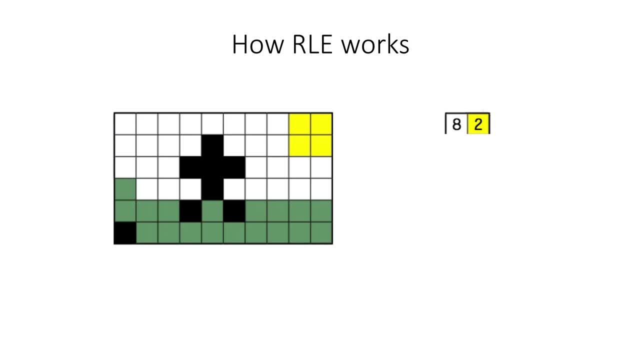 this is what it looks like. so you have eight white pixels and you have two yellow pixels. so if we just write them down like this, then the next row, if you look at the next scan line, which is 4 white, 1 black, 3 white and 2 yellow, then 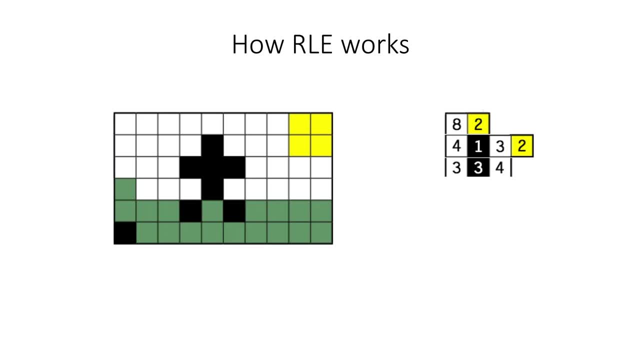 the next one is 3 white, 3 black and 4 white, and the next one is 1 green, 3 white, 1 black and 5 white. Then the next scan line is 3 green, 1 black, 1 green, 1 black and 4 green. 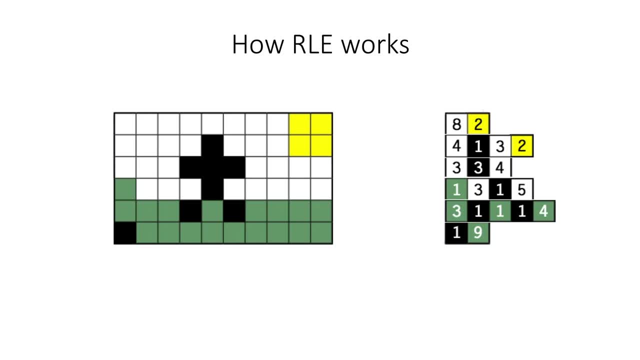 And the last line is we have only 1 black in the beginning and then 9 green pixels. So this is how this image actually looks like if you code it in that order. Now this: if you calculate, you got 16 bit, which means if you represent the number of time. 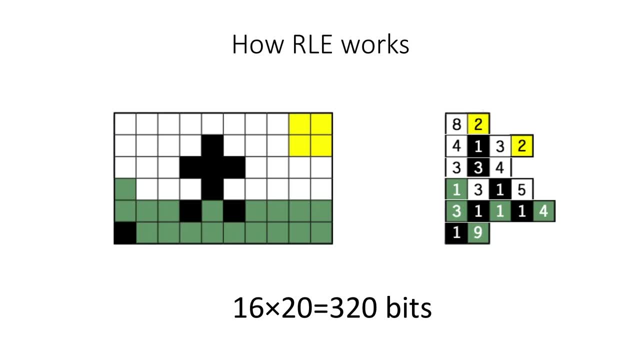 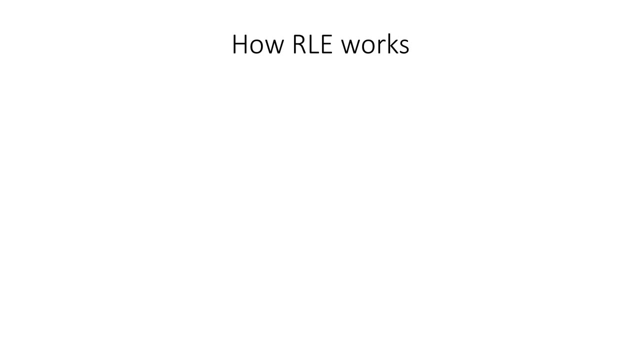 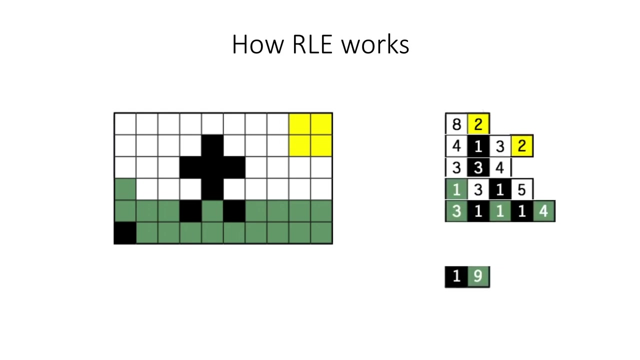 it occurs, which is 8, you can store that using 8 bits, and then the color is white, which is another 8 bits. that will represent 16 bits. So 16 times 20, which is 320.. Ok, so if we look at this image, this can be also represented in a data pair. 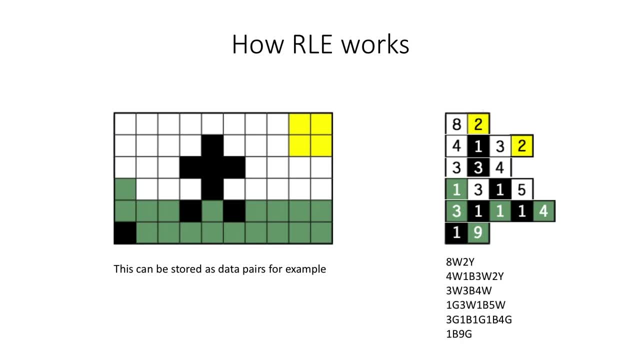 So what do I mean by data pair? well, you can actually store this in this way. If you look at this first, we have 8 white, so we can represent that saying 8w, w for white, 8, 8 occurrence and w for white.